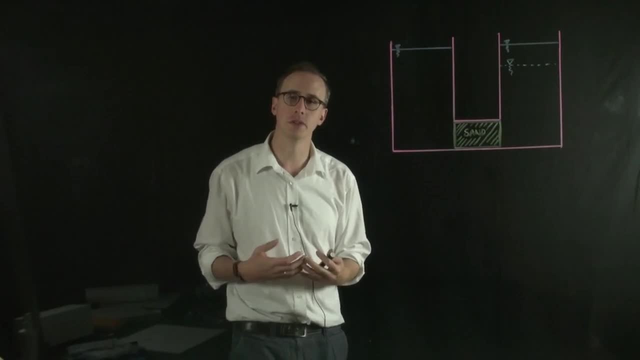 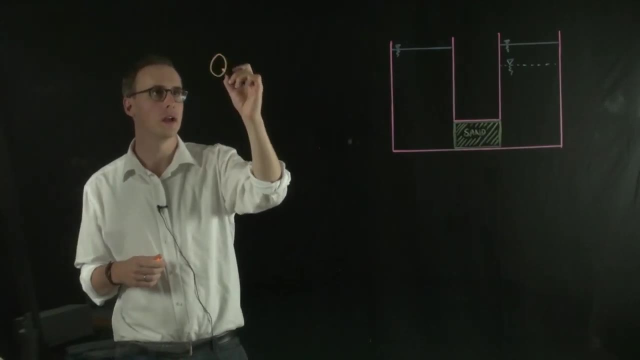 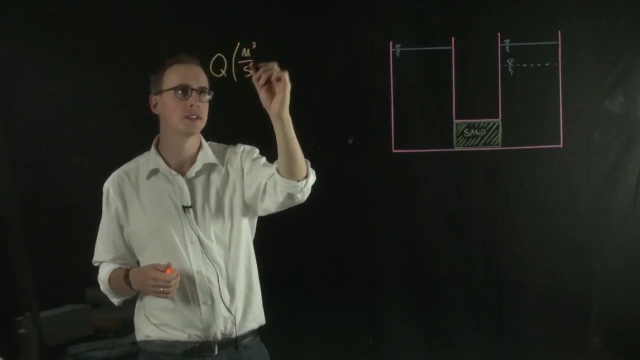 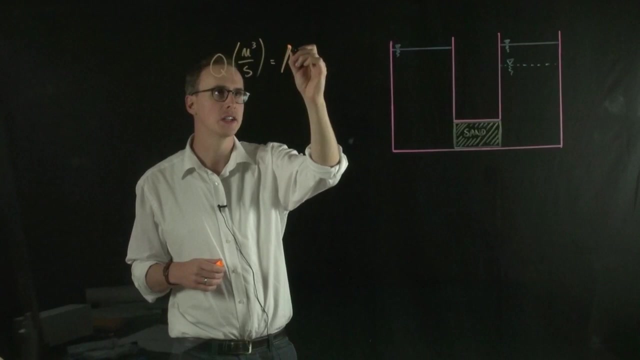 which relates or is an equation for the flow of water through the material. So D'Arcy's Law says something about flow, and that's q And that's flow of water, so meters cubed per second say, And it says that this flow is equal to the cross-sectional. 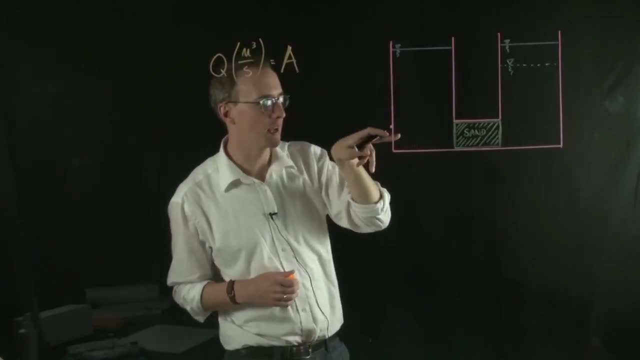 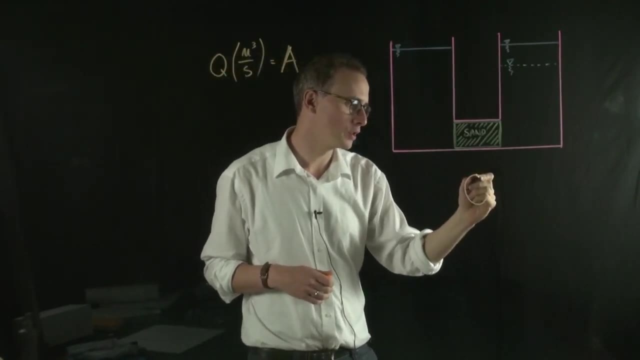 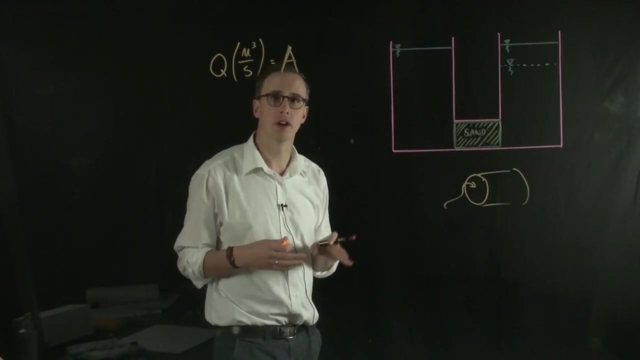 area of the flow. So in this case, if we were looking at the sand in this direction and if it was a round tube, we might be looking at a tube that looks something like this. So D'Arcy's Law is interested in the cross-sectional area of the flow path, So it would be this: 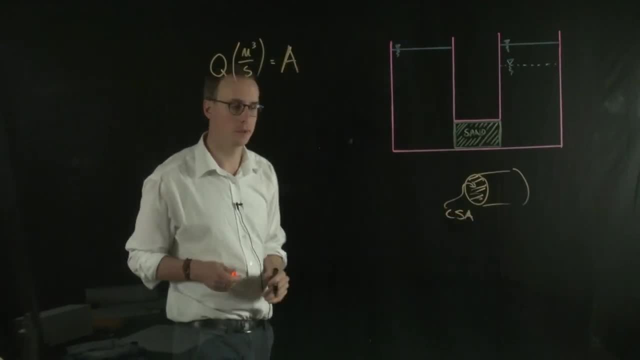 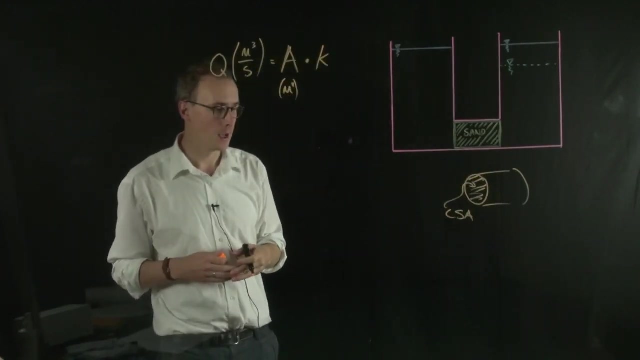 cross-sectional area in this example, And that has units of meters squared, And then we then multiply that by the permeability. So what the permeability says is how susceptible this material is And that's for water flow through it, And that is given the units of meters per second. 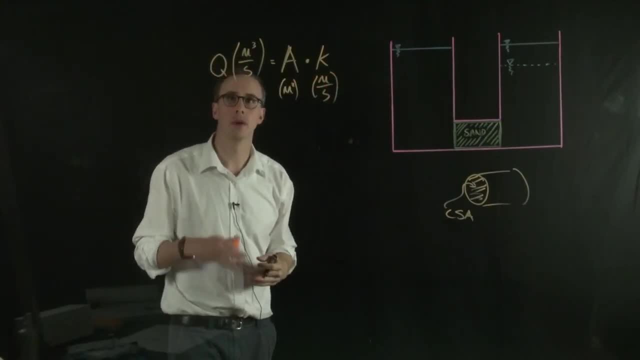 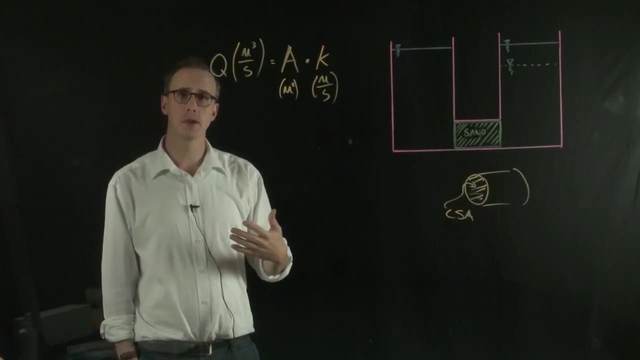 So you can see, if we multiply these two units together, we'll get our units of flow. So when we talk about permeability, we often talk about it on a log scale, And that's so we can cover a huge range of different permeabilities that materials have. So something like a clay. 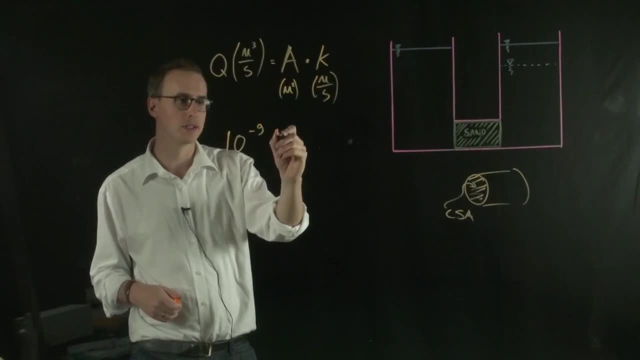 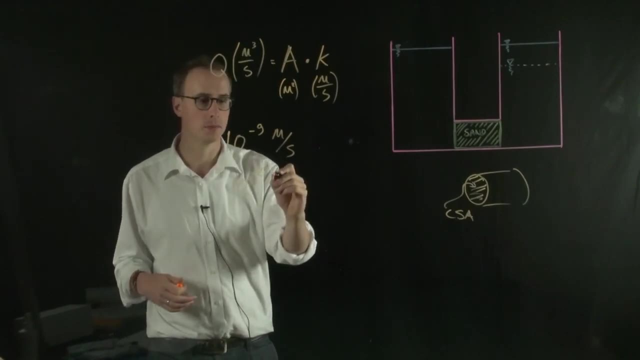 might have a permeability on the order of 10 to the minus 9 meters per second, Whereas a sand or a gravel might be on the order of 10 to the minus 2 or something meters per second. And you can see that we've got seven orders of magnitude. It's 10 million times. 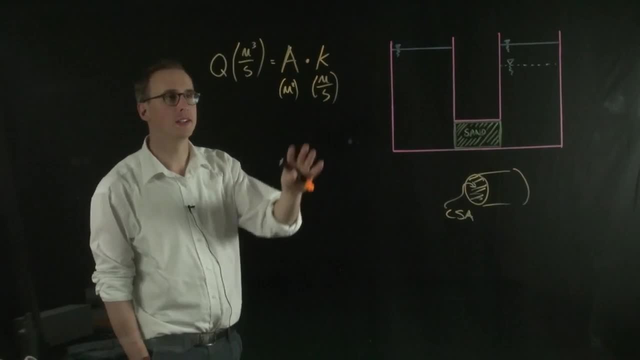 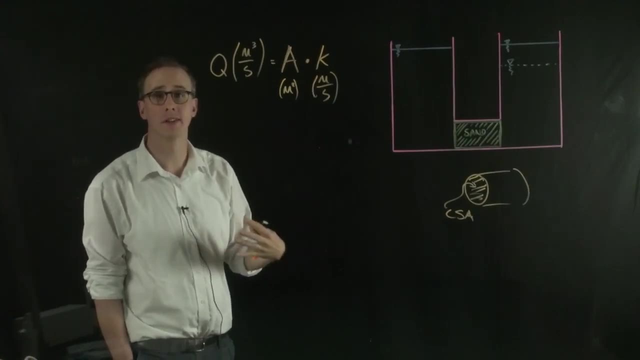 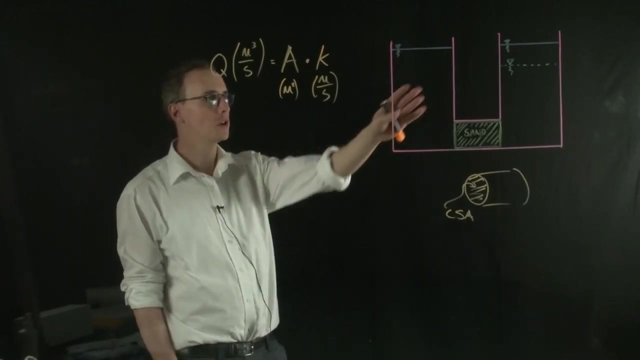 different in permeability. So what this equation needs now is some sort of driving force. to talk about flow, You can say that we've got a cross-sectional area and a permeability, And those are both specific to the soil that we're looking at. But we need a driving force. So what drives the flow? 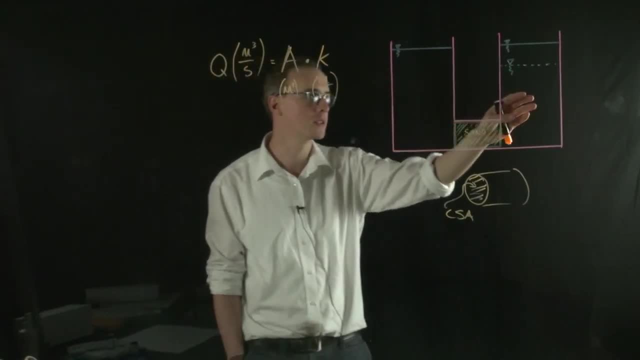 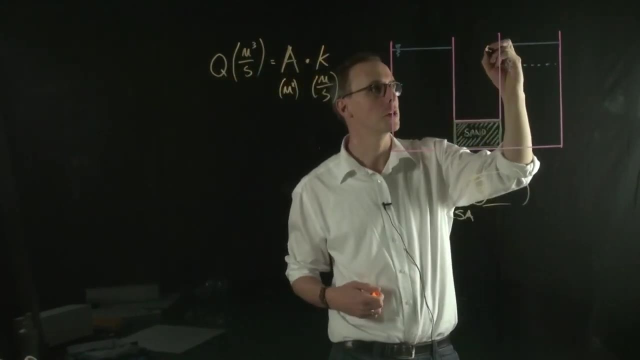 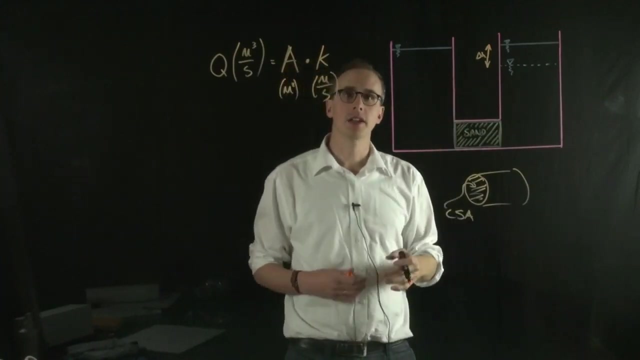 of water from this side of the area. So this is the system to this side And it's the difference between the levels of water. So delta H in this case, And you can see that if we had a larger delta H, we'd have more.